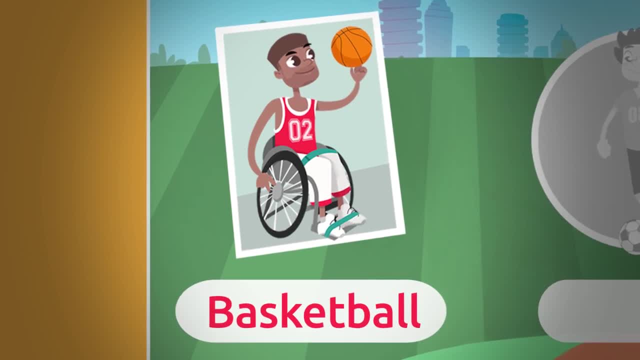 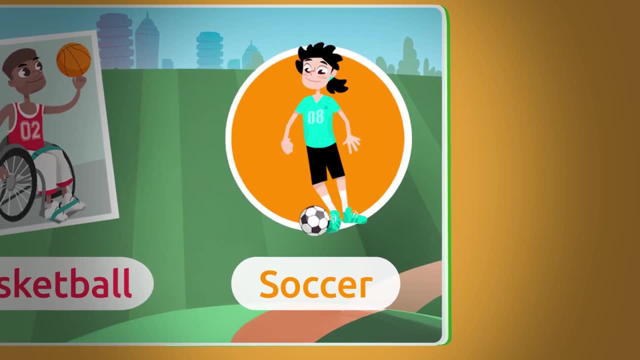 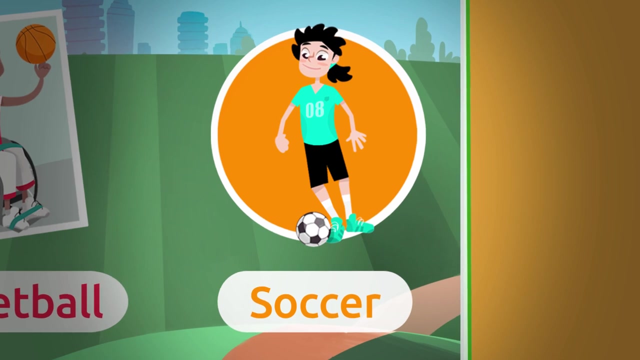 To move, you need to bounce the ball. Basketball: This is a soccer sticker. In soccer, the winning team is the one that gets the ball over the opposing team goal line more times. You can kick or head the ball- only Soccer. 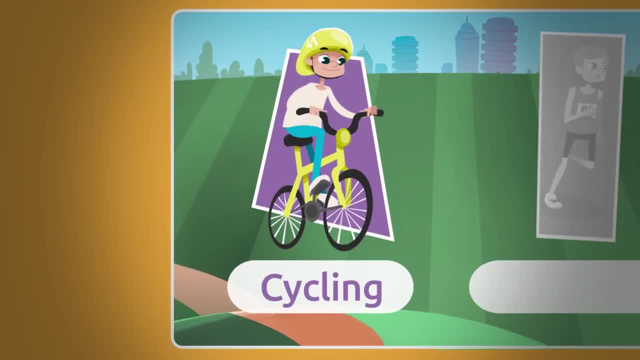 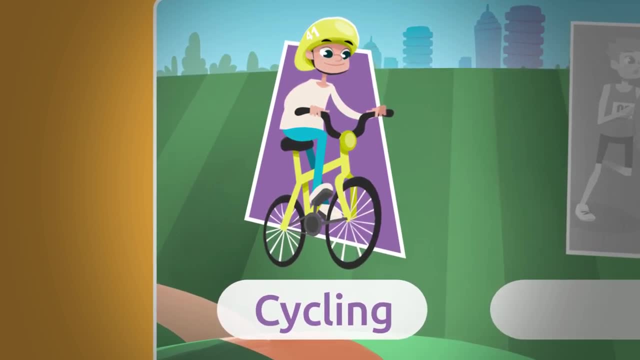 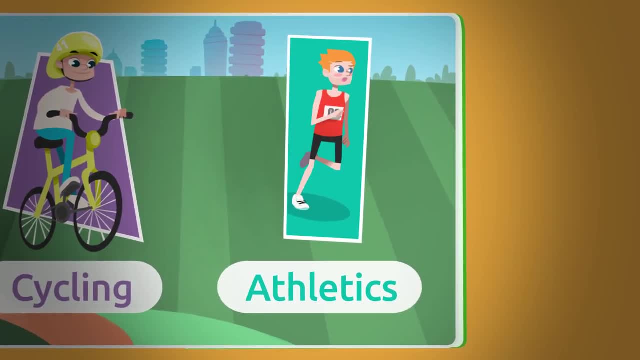 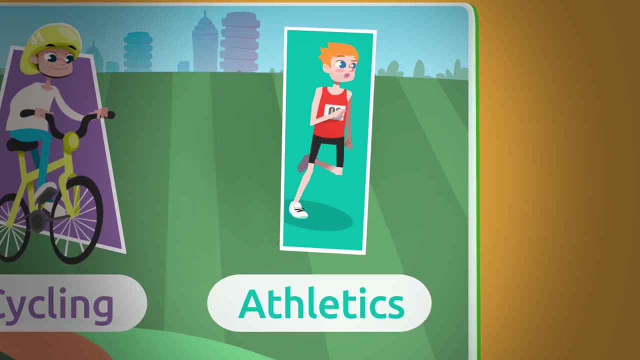 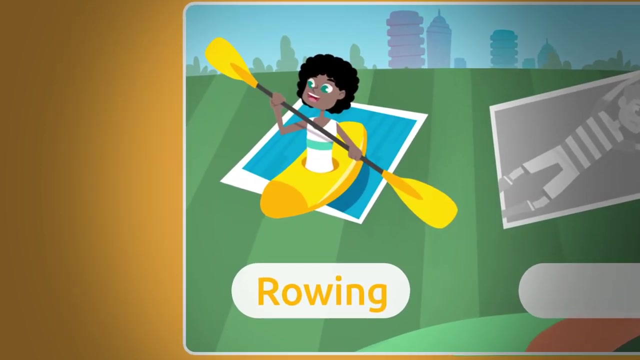 Let's see what else we have here: Athletics. Athletics is a group of sport activities like sprint running, jumping and throwing Athletics. The next one is a rowing sticker. In this sport, rowers propel a boat on water using oars. 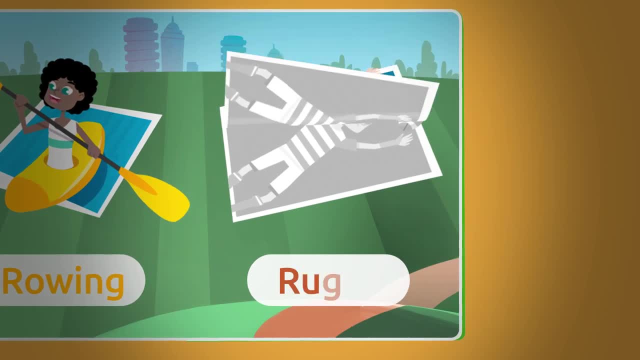 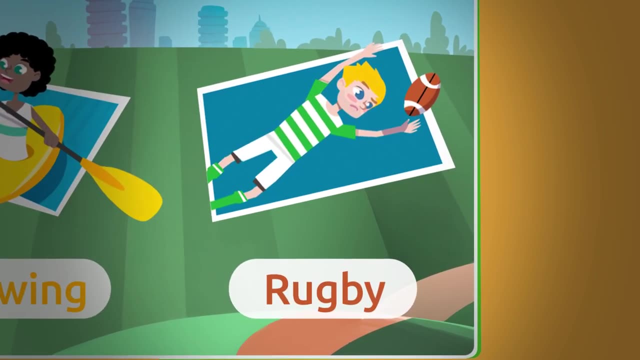 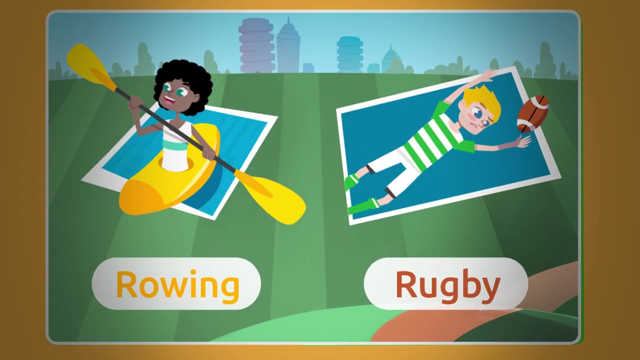 Rowing, And this is a rugby sticker. Rugby is played by two teams that have to compete in a game. The first team has to carry the ball to the opponent's end of the field. The ball is oval shaped Rugby. Let's see this next one. 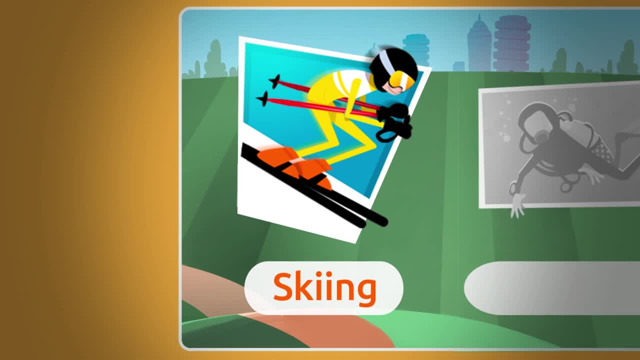 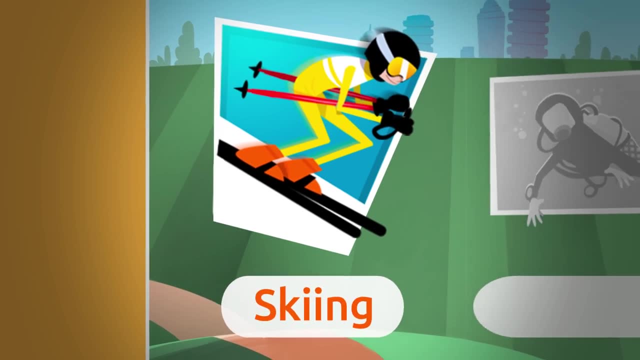 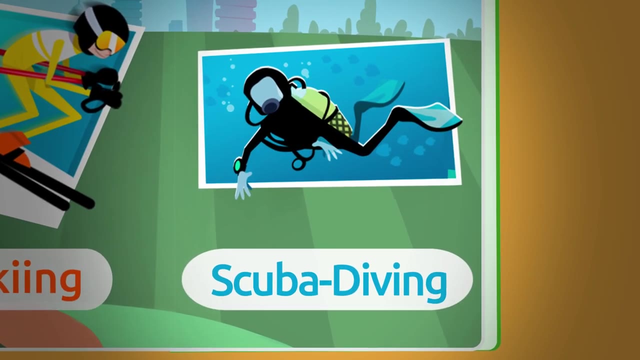 A skiing sticker To ski skiers slide on snow using skis that are long boards fixed on their feet Skiing. And the last sticker is a scuba diving sticker. Scuba diving is practiced underwater. You use goggles, diving flippers and a diving tank. 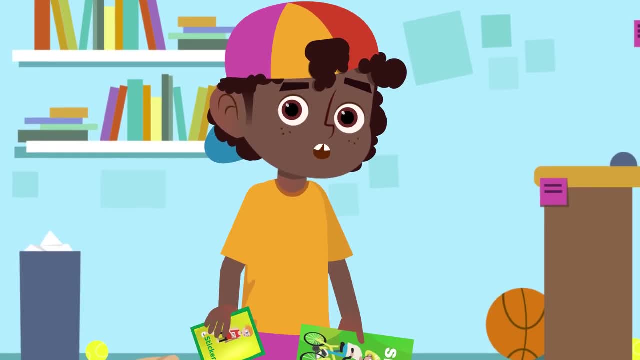 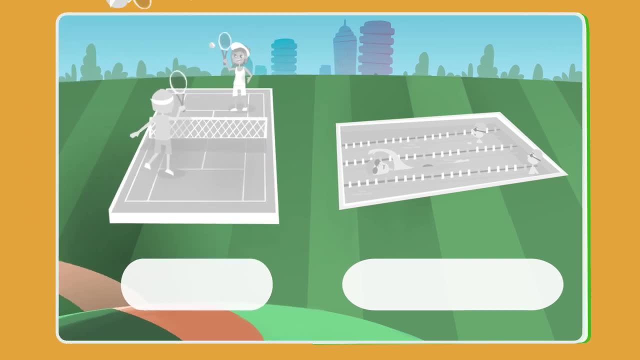 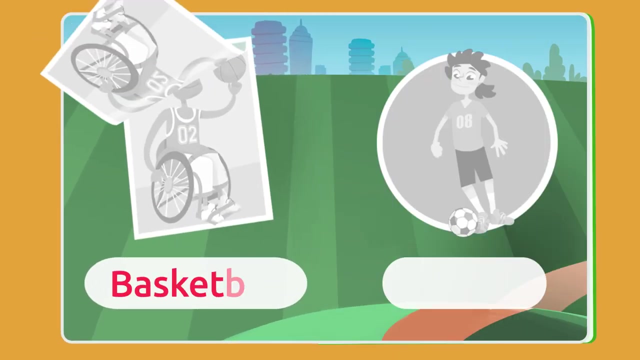 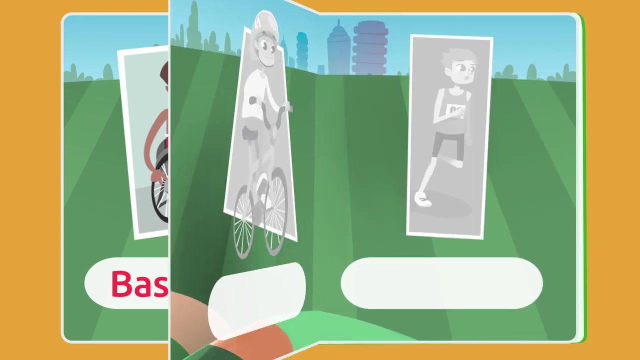 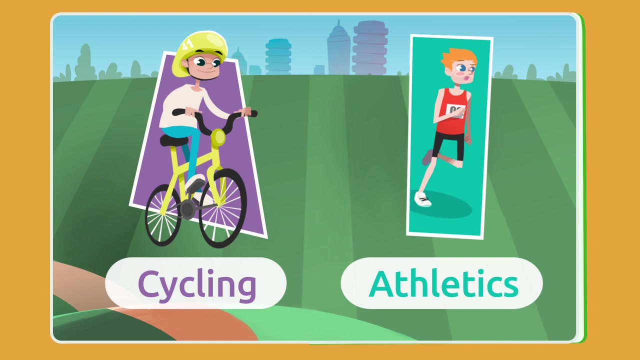 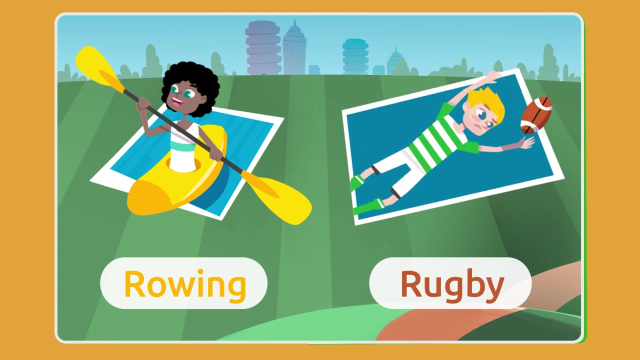 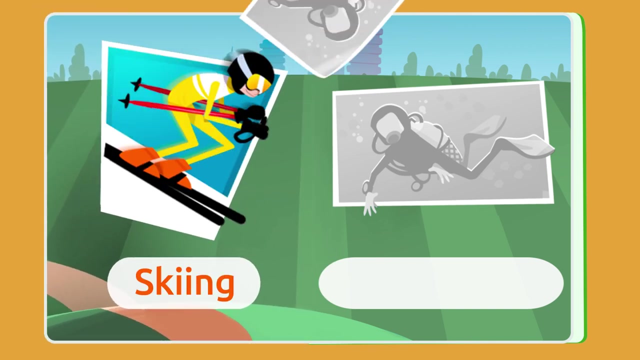 Scuba diving. We learned so many sports words today. Shall we recap them: Tennis, Swimming, Basketball, Soccer, Cycling, Athletics, Rowing, Rugby, Skiing, Scuba diving. How amazing. Well, I still have to finish putting the stickers in the stolen bags.